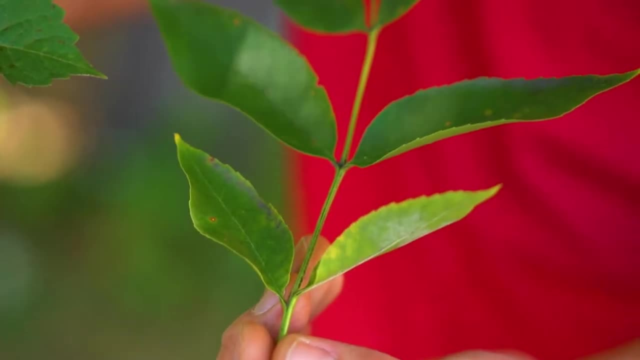 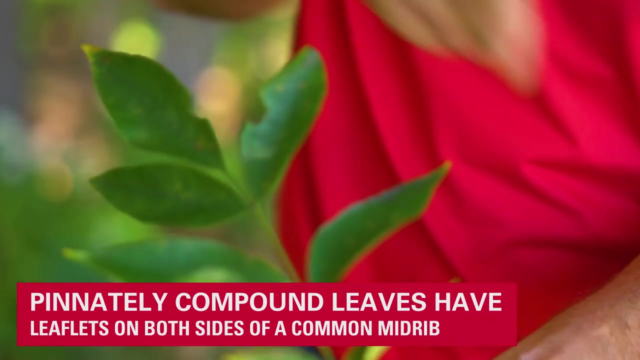 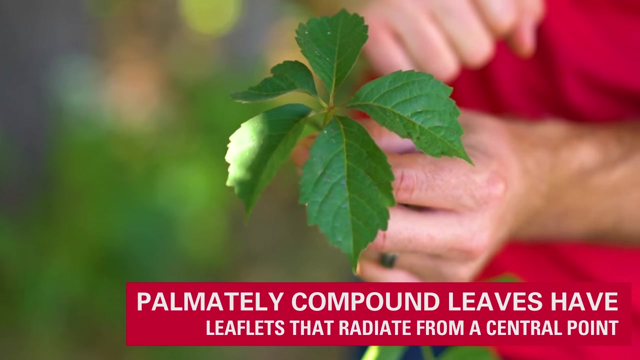 be broken down further into pinnately compound and palmately compound. Pinnately compound leaves such as this green ash have leaflets arranged on both sides of a common midrib. Palmately compound leaves such as this Virginia creeper have leaflets that radiate from a central point Like a family. 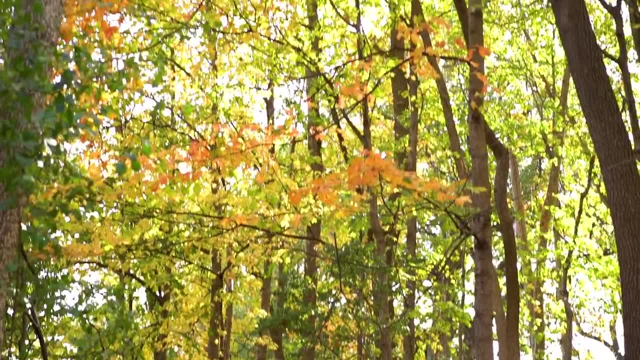 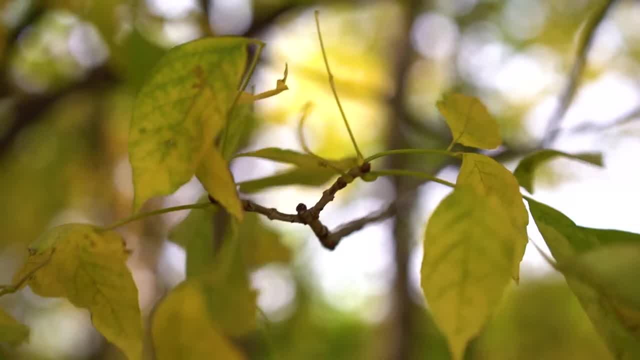 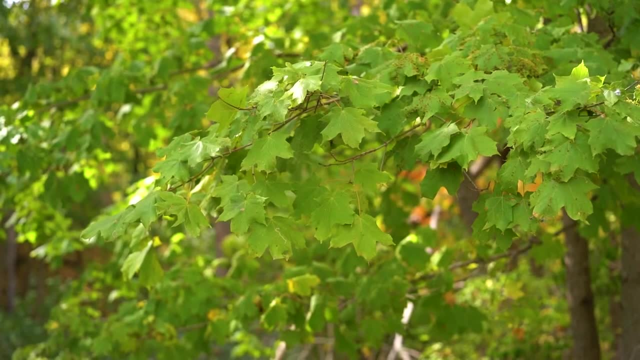 they have a good amount of leaflets. The overall shape and relative size of the leaves or leaflets are also key identifying characteristics. There are many leaf shapes in the Iowa woods. However, I recommend you become familiar with some of the more recognizable shapes first. 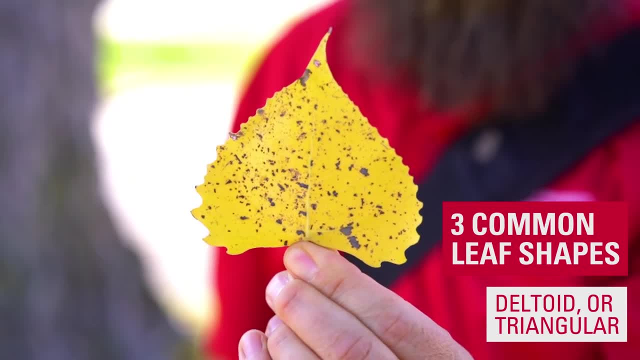 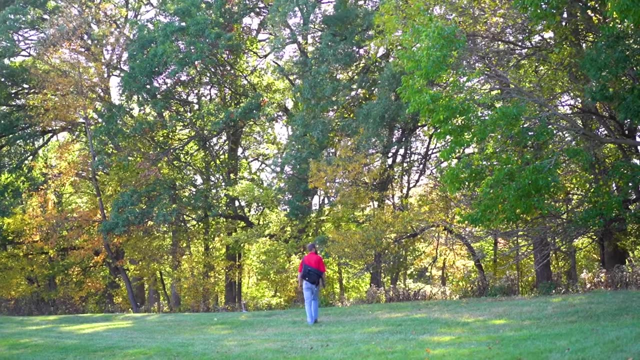 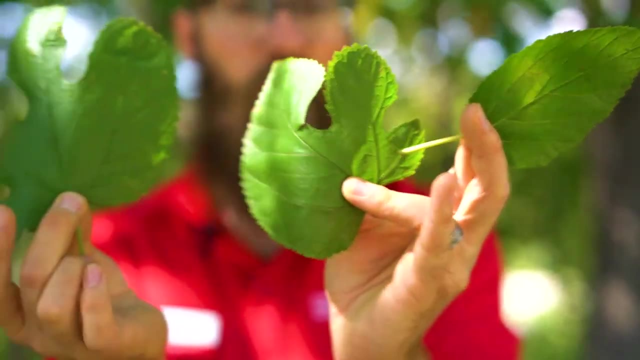 These include deltoid or triangular, chordate or heart-shaped, and lanceolate or lance-shaped. Watch out, though, because certain species, such as white mulberry, often have two or three distinct leaf shapes on the same tree, So check multiple leaves on each tree you encounter. 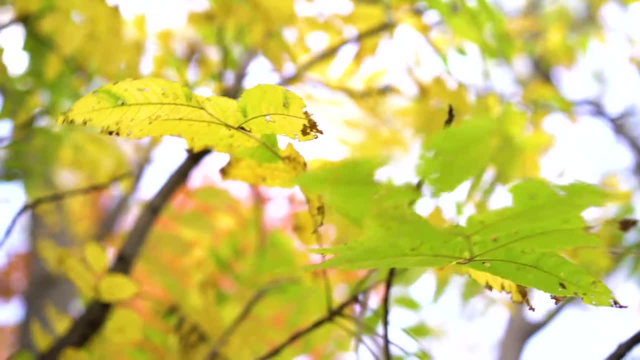 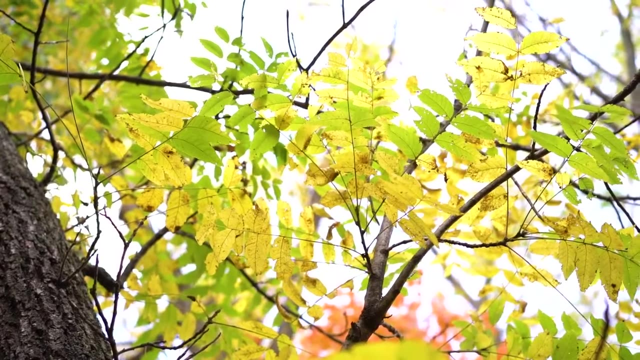 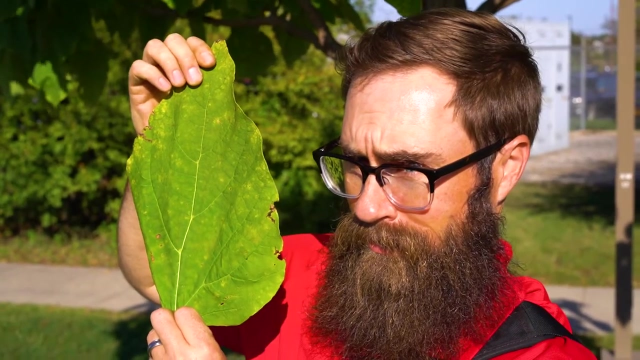 Leaf size ranges widely too. Using leaf size for ID can be tricky, as size may vary within the same species and even within the same tree. However, some species like sycamore and catalpa are notorious for producing leaves of epic proportions. My third identifying feature for leaves is the leaf. 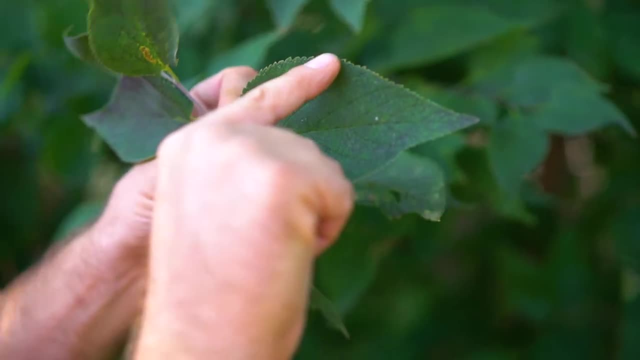 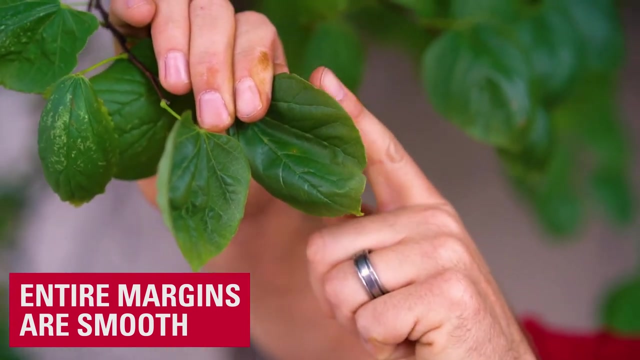 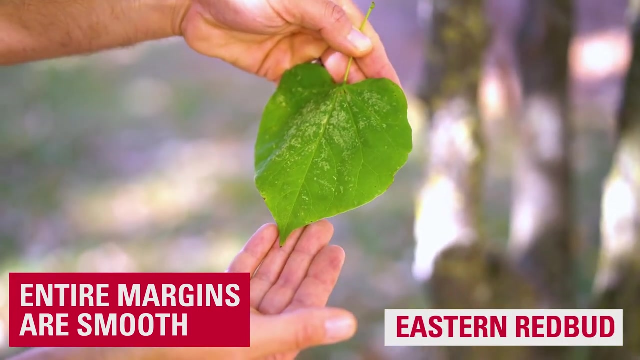 margin or the edge of the leaf blade. The first thing to assess is whether the leaf margin is entire. Entire margins are essentially smooth, meaning they lack serrations, notches or other divisions, such as this eastern redbud, Like shape and size. you'll see an exciting range of leaf margins in the Iowa woods. 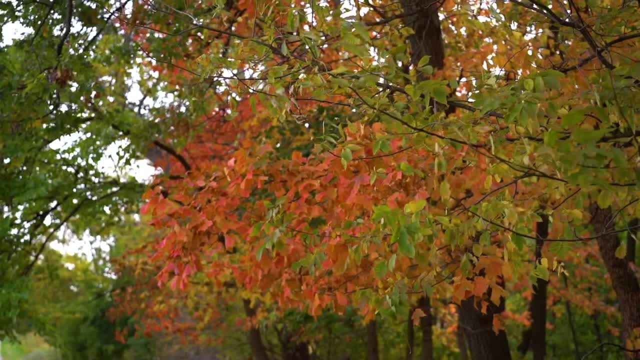 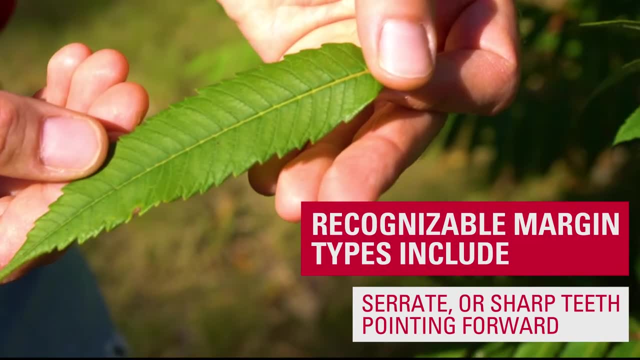 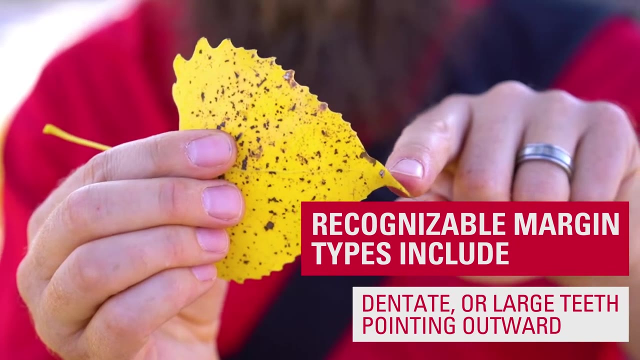 As before, I recommend you become familiar with some of the more recognizable margin types. first, These include serrate or having sharp teeth pointed forward. dentate or having large teeth pointing outward. sinuate or wavy, and lobed or divided into segments.